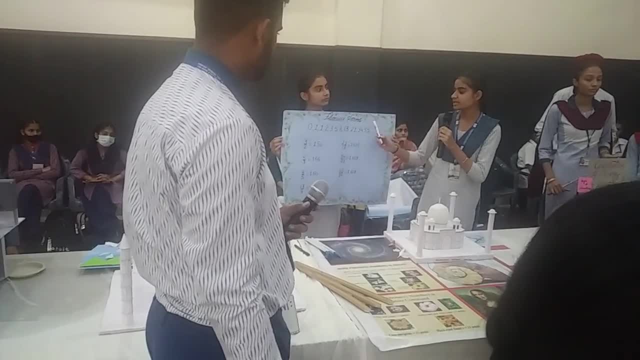 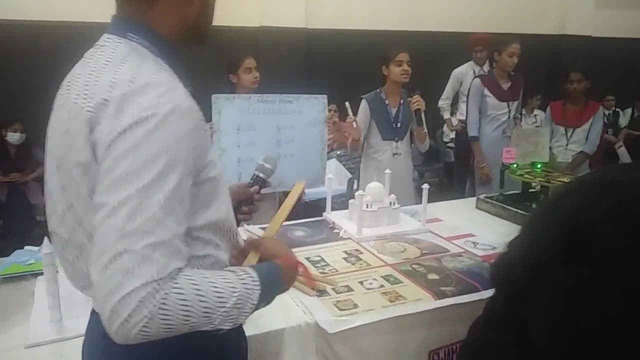 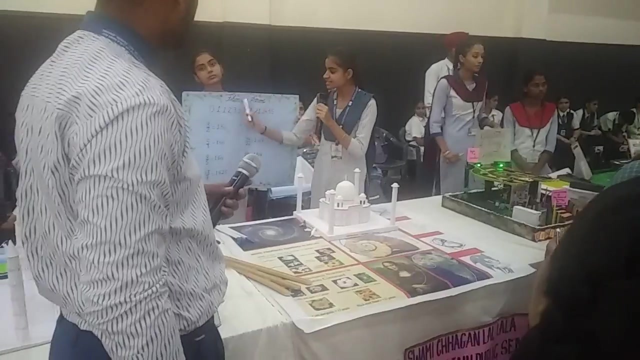 Moving further, 13 plus 8 gives us 21,. 34 plus 21 gives us 55, and so on. Now this pattern holds a very powerful secret of nature: How? Let me tell you Now, if I take each number. 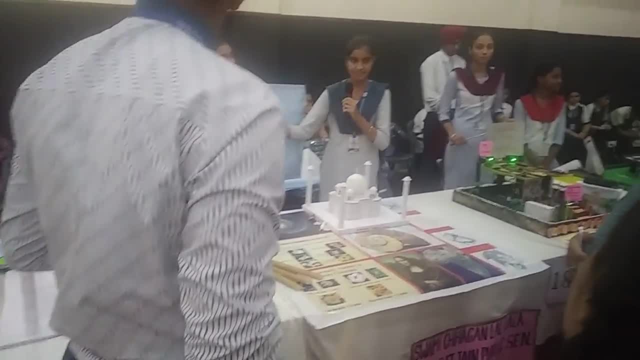 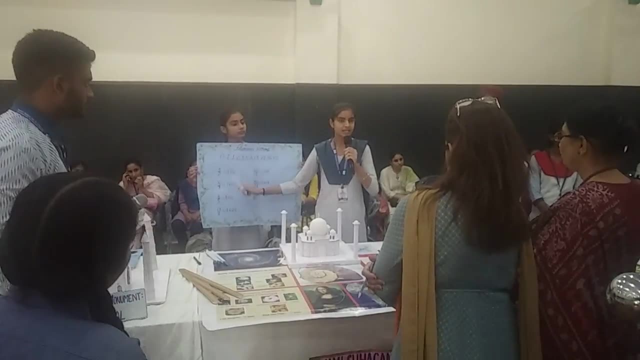 In the series and divide it by its predecessor. Like, if I divide 3 by 2, I will get 1.50.. If I divide 5 by 3, I will get 1.60.. If I divide 8 by 5, I will get 1.60. 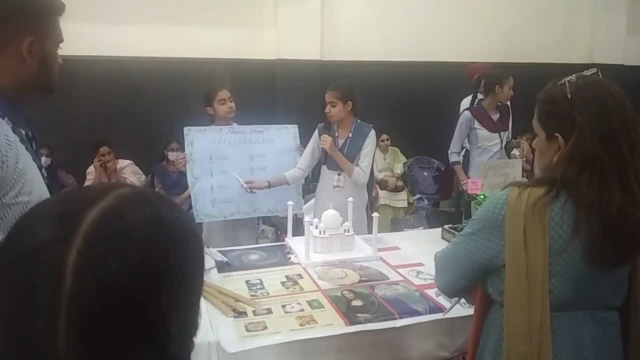 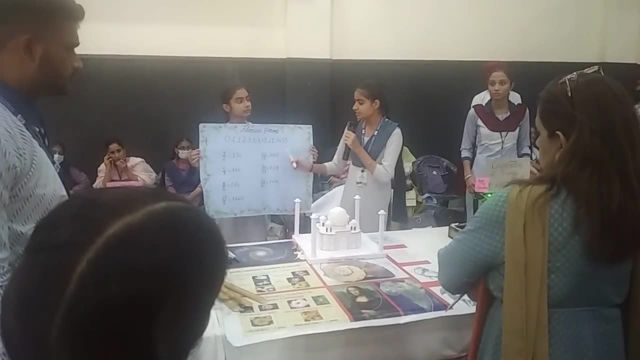 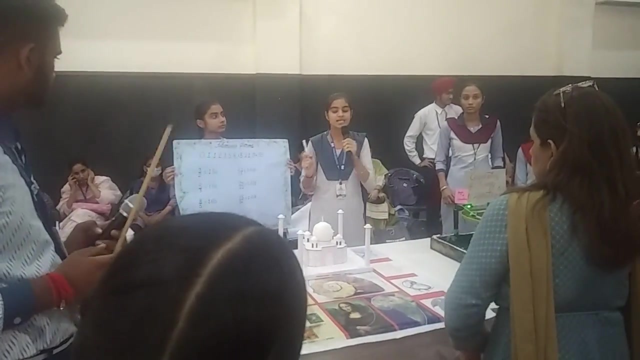 Moving further, if I divide 13 by 8, I will get 1.625.. If I divide 21 by 13,, I will get 1.615.. Next, if I divide 34 by 24.. I will get 1.615. and, last but not least, if I divide 55 by 34, I will get 1.617. 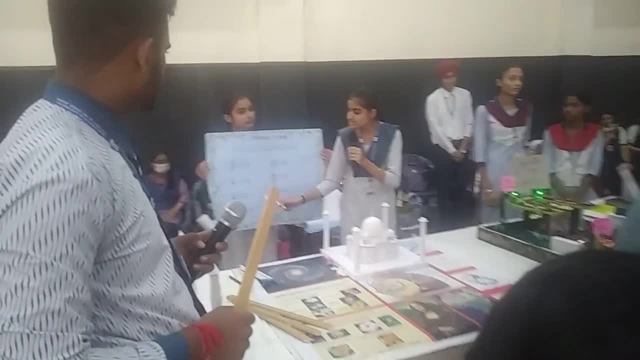 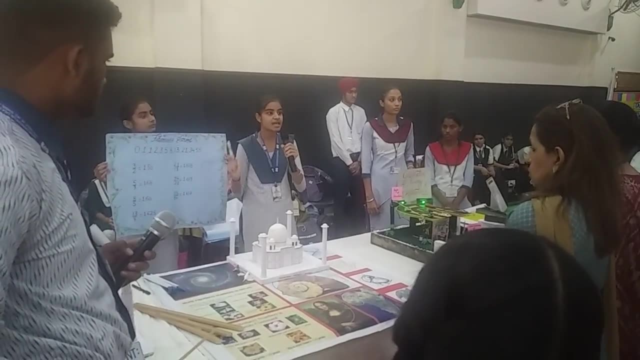 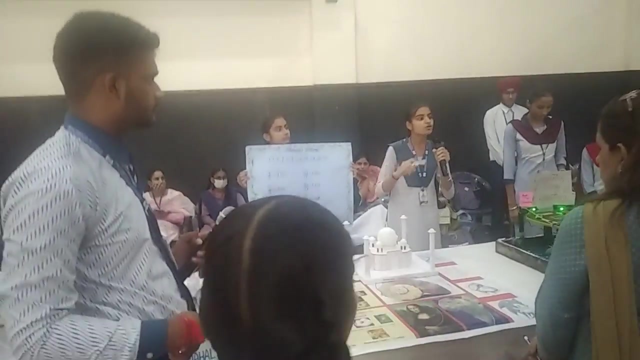 Now you will observe that we are getting a constant value where the ratio 55 by 34, which gives us 1.617, is nothing but the famous golden ratio which has fascinated mathematicians and scientists from all over the world. Now my companion, 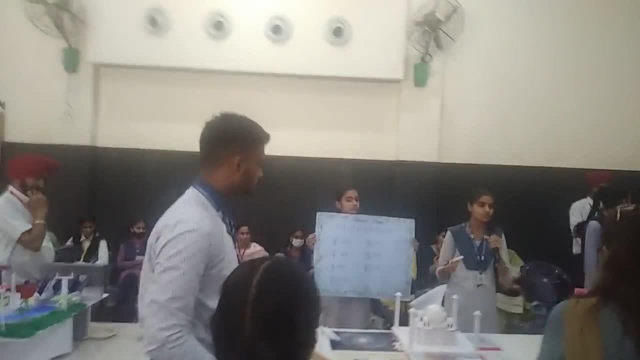 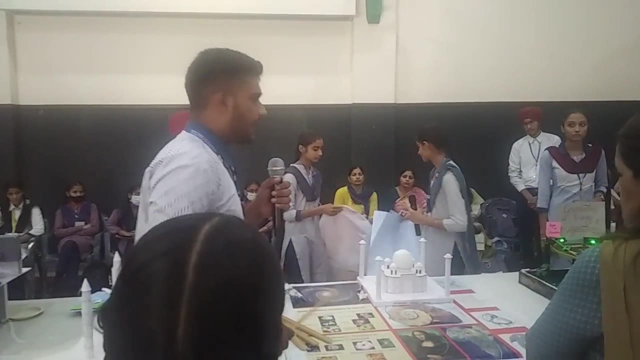 Let's hear you further about the golden ratio, and it's used in the field of science. Thank you, Fibonacci numbers, the magic of numbers. The secrets of these numbers are 0, 1, 2, 1, 2, 3 and so on. 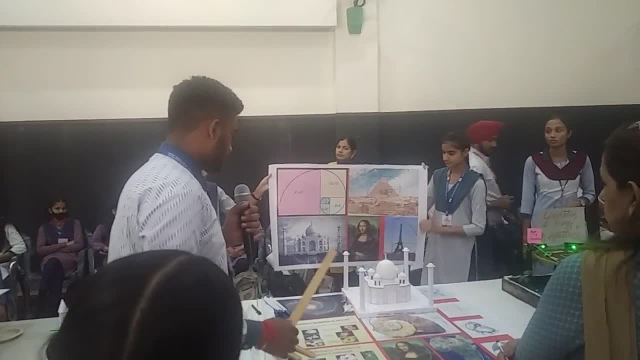 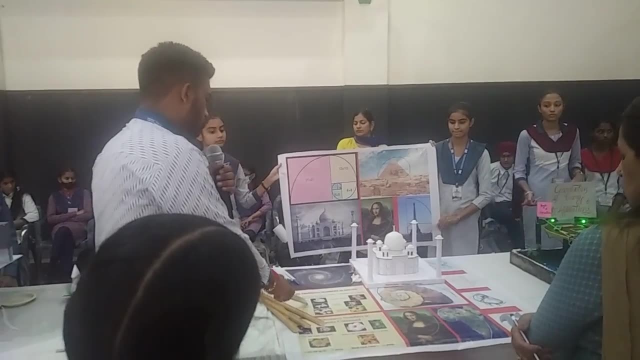 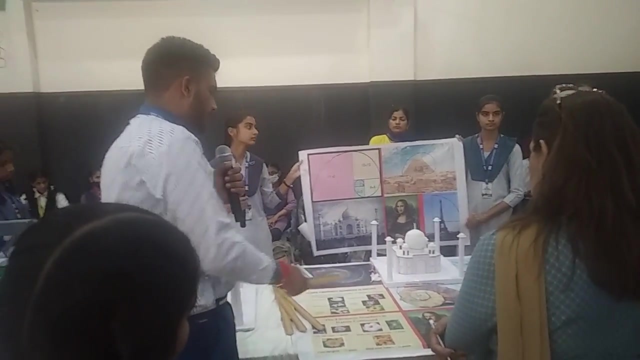 The number of these numbers can be seen in patterns. The patterns of class are arranged in Fibonacci numbers. Like, we have a number of the number: The number of patterns in the legal science, The number of patterns in the legal history, The number of patterns in the legal history and so on, like in the forbearance. 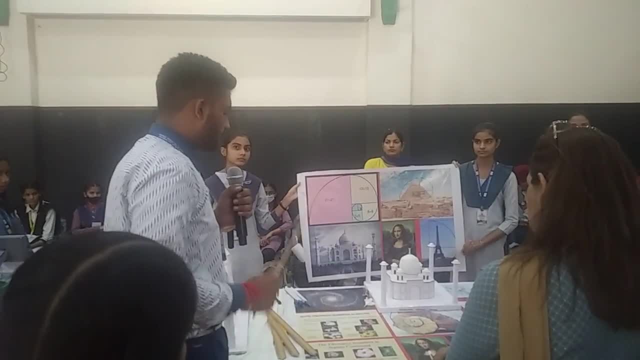 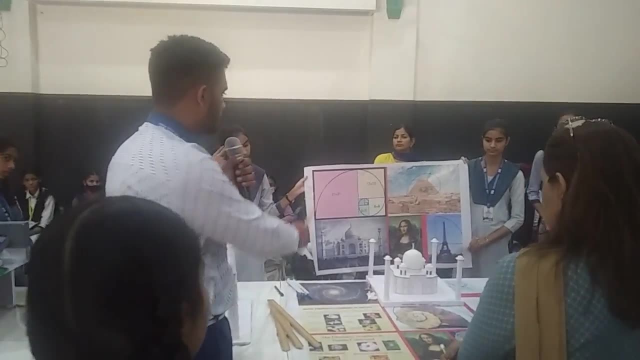 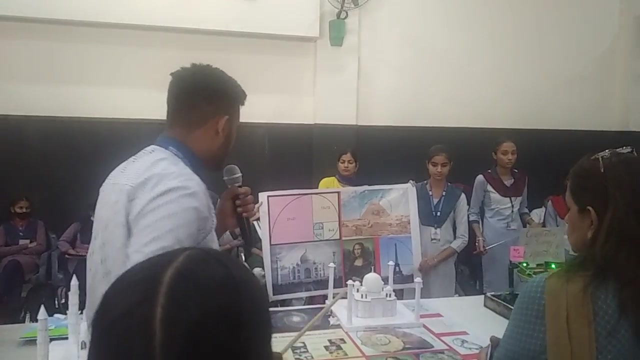 These all are Fibonacci numbers. Fibonacci numbers, if arranged, the scale of these numbers, if arranged accordingly, makes a spiral, the golden spiral. The shape of this spiral is same as that of all the spirals in this universe, Like the shape of the galaxy, shape of shell, the component of rica, sonic heart. 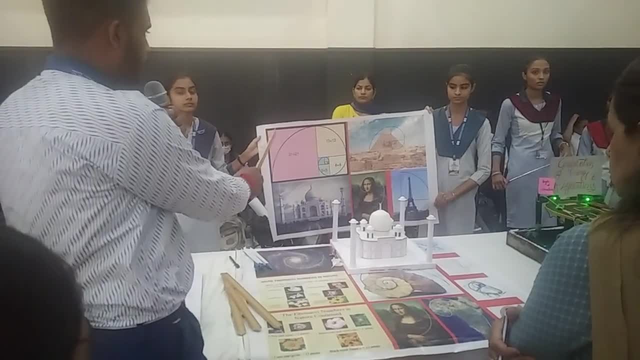 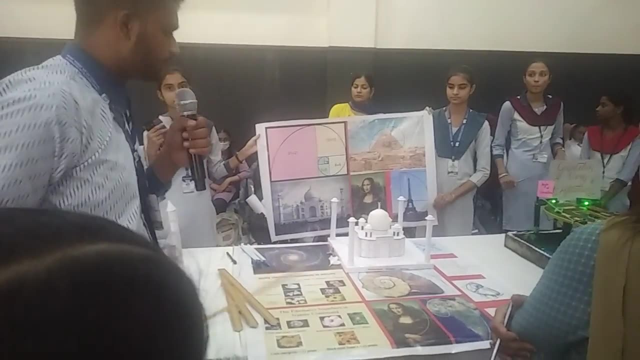 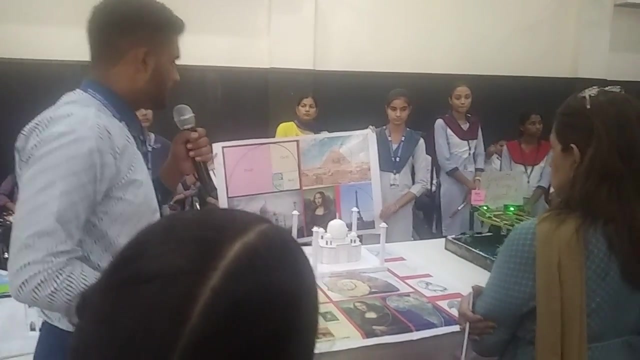 It is monoisomatic. It all resembles with the shape of golden spiral. Almost all the spirals in this universe have the shape resemblance with this golden spiral, Golden ratio, A ratio which shows almost all the dimensions and integers. The ratio is 5 by 1.. 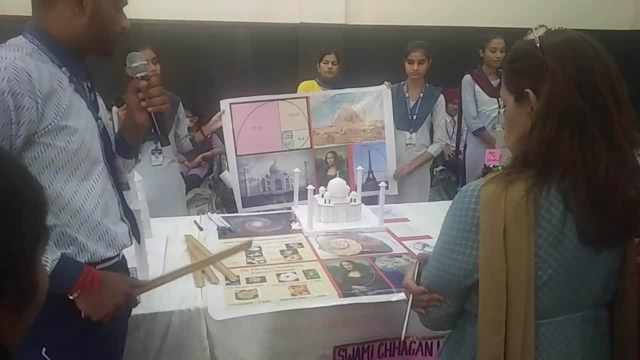 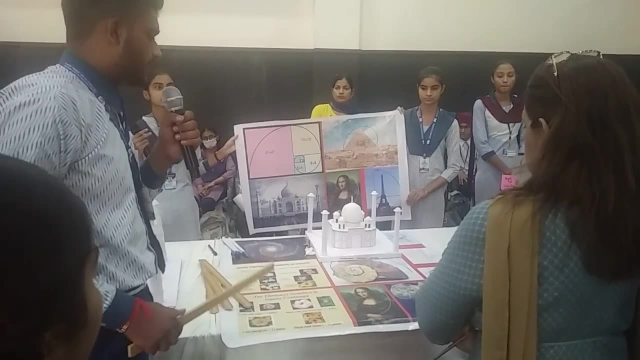 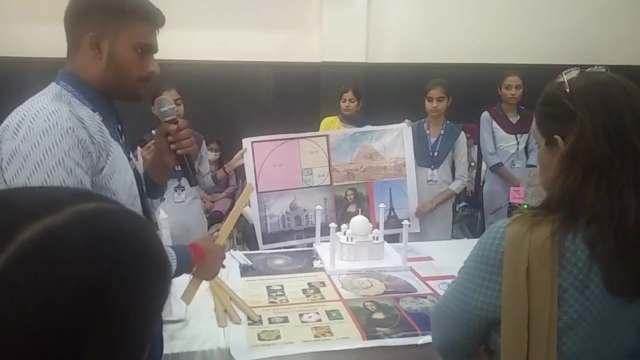 5 is an international number with approximately value of 1.618, as same as that of golden ratio. Monuments, objects or building. Monuments, objects or building: All that can be divided is divided in this golden ratio. The Fibonacci proximity numbers, if divided, give the same ratio as that of golden ratio. 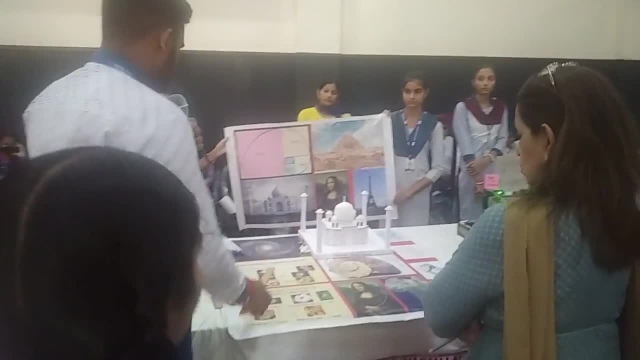 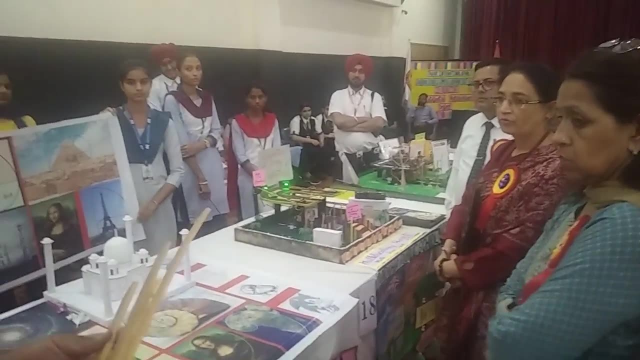 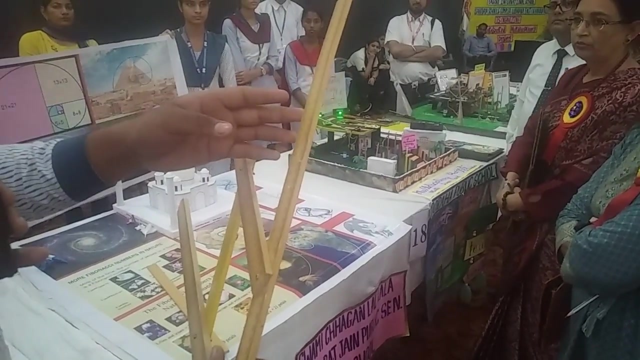 This phenomenon can be seen in all the objects in our surrounding. The golden ratio can best be associated with the help of this golden caliber. This golden caliber is made with the help of four scales arranged like a star in a circle. One ratio of golden caliper tells us about 1.6 part, and second ratio of 1 part. 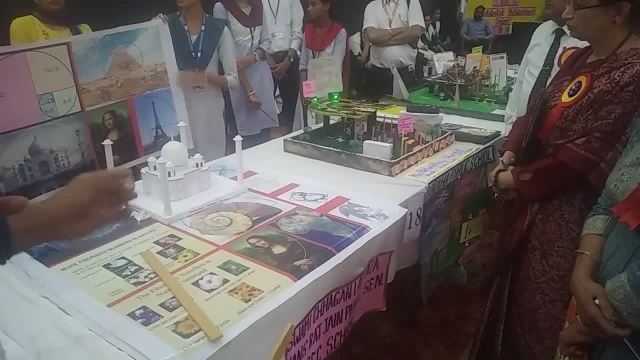 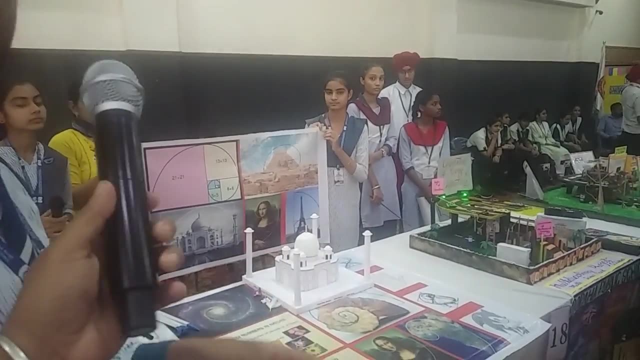 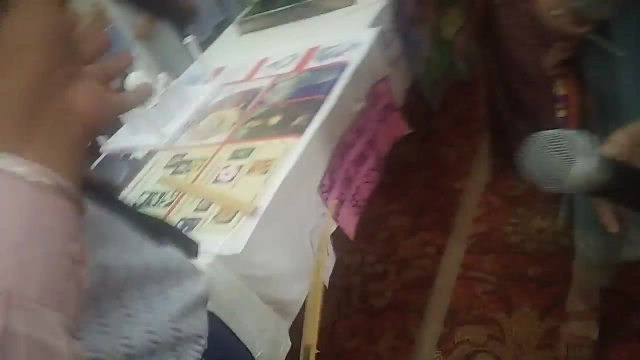 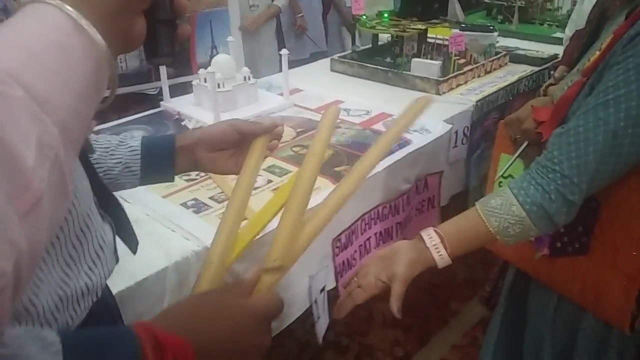 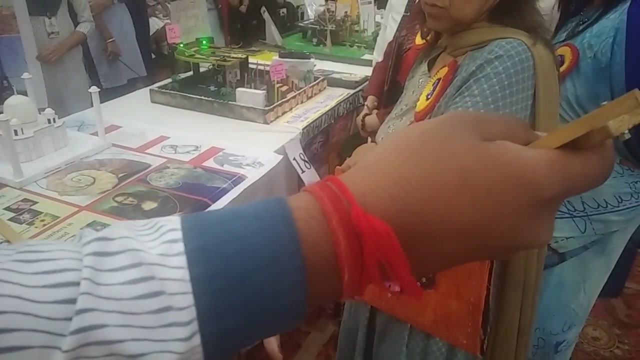 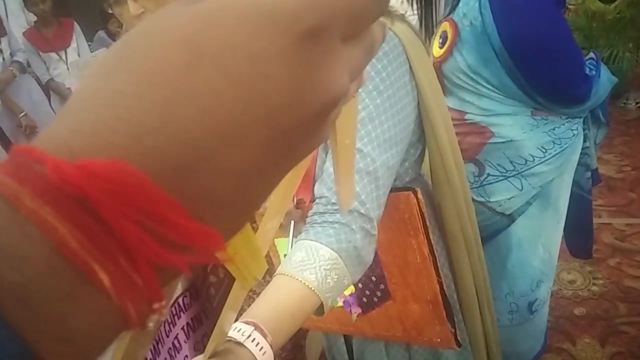 This ratio can also be seen in human DNA. The ratio of length of segment of one DNA is 1.618, as same as that of the golden ratio. This ratio can also be seen in a human head. The ratio from length of the elbow to wrist by the hand is 1.618.. 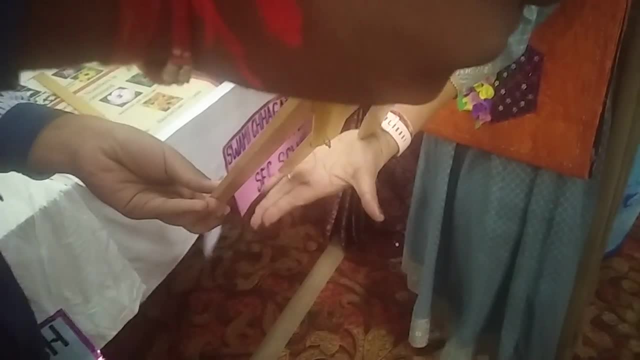 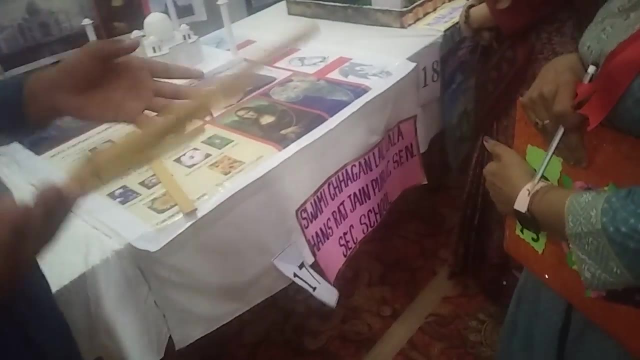 And also of the fist of the hand. If we take from wrist to fingers by finger, it is 1.9 fist. It can also be seen in a finger, Like from forehead to eyes, by eye to chin, it is 1.5 fist. 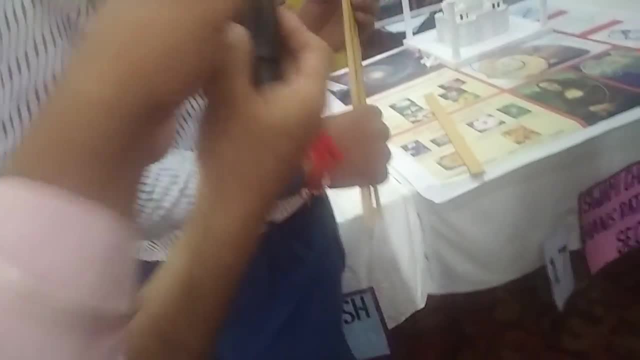 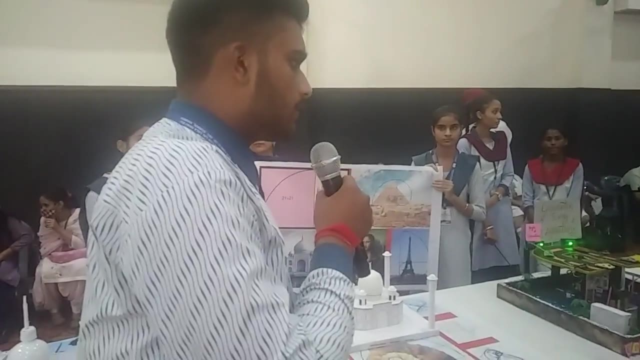 Can you show me the chart of the first look of the first jump? Imagine the first look of the first jump. Like in monuments, there is also golden ratio used. Can you see? also Like in the, It is used for construction somewhere. 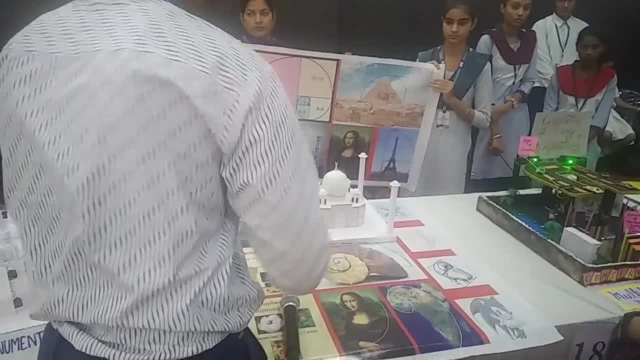 Which construction? Which one? Taj Mahal, Taj Mahal, Which one? Taj Mahal, Taj Mahal, Taj Mahal. Now we get about ABS box size. Looking at Orchard zone, there is a box size that looks like a Ilona box size.